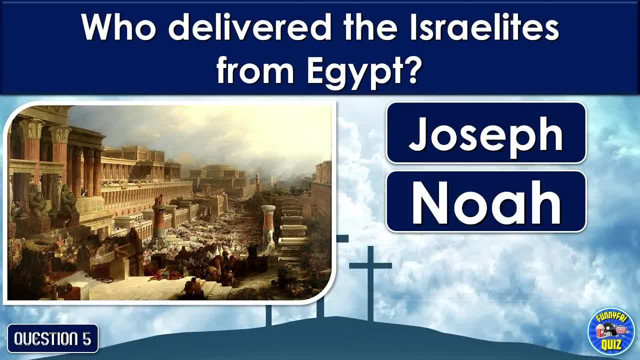 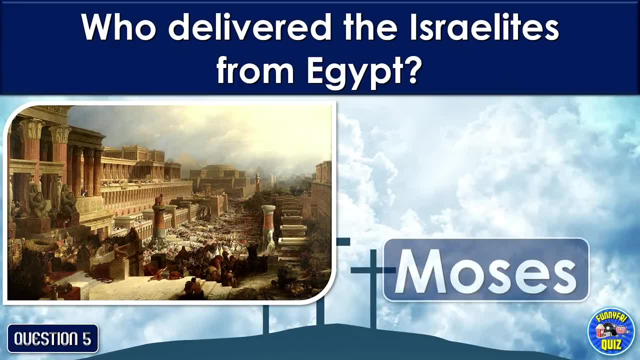 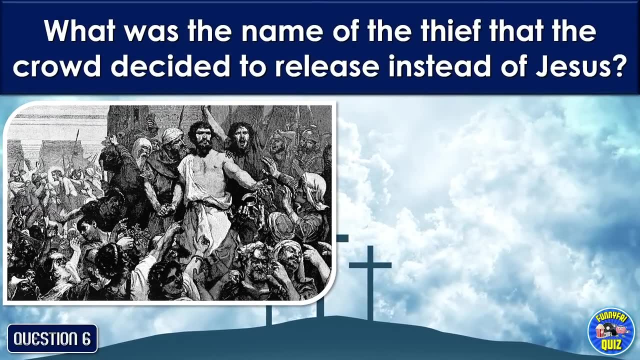 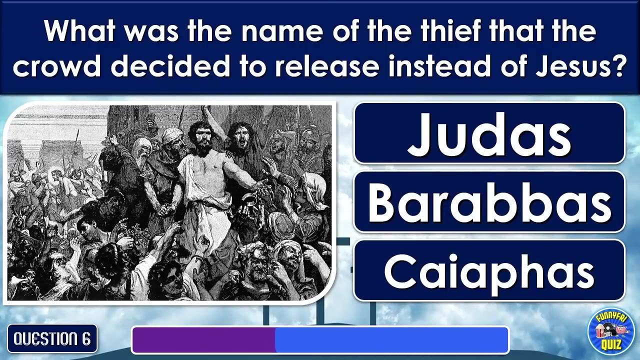 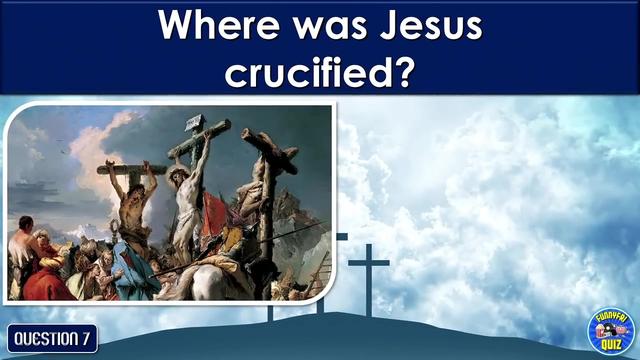 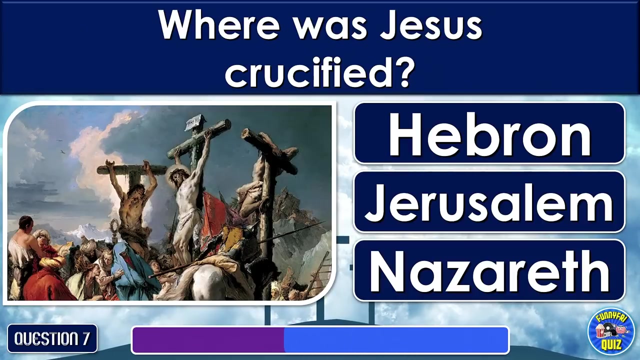 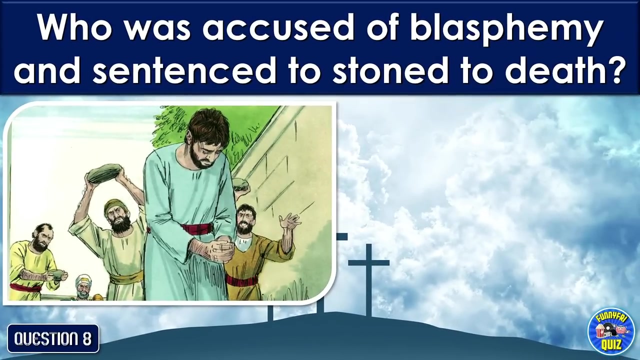 The Israelites from Egypt? Moses, What was the name of the thief that the crowd decided to release instead of Jesus Barabbas? Where was Jesus crucified In Jerusalem, Who was accused of blasphemy and sentenced to stone, to death? 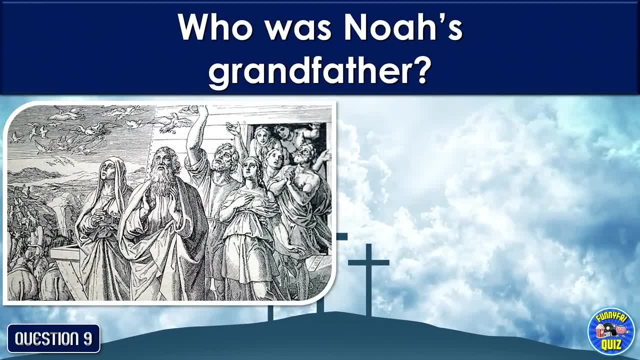 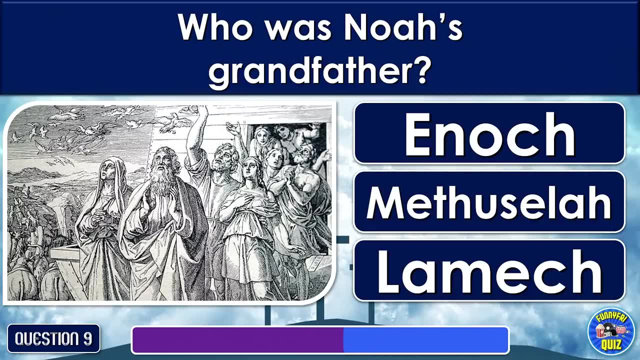 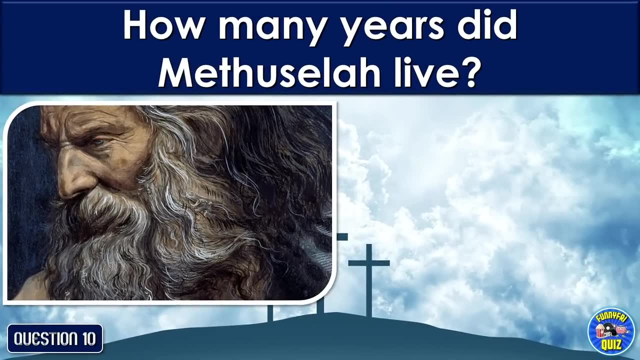 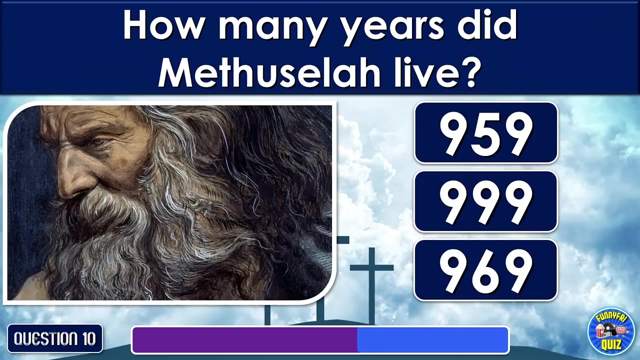 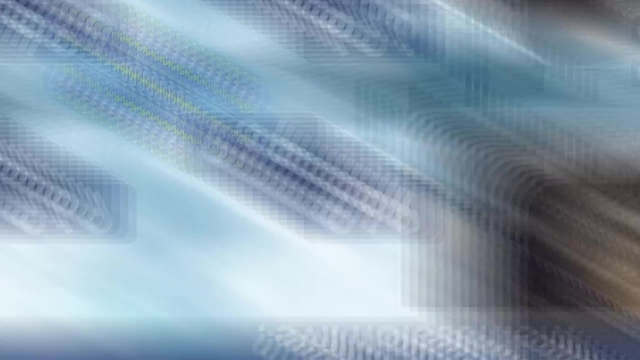 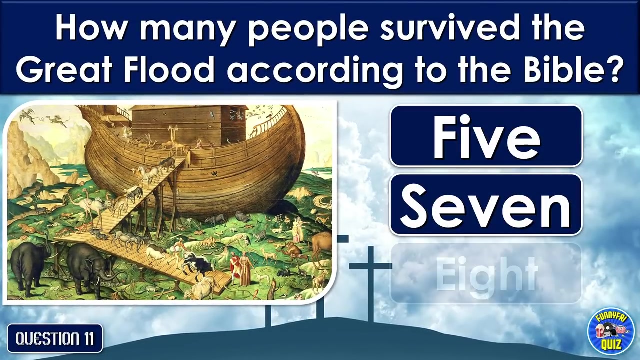 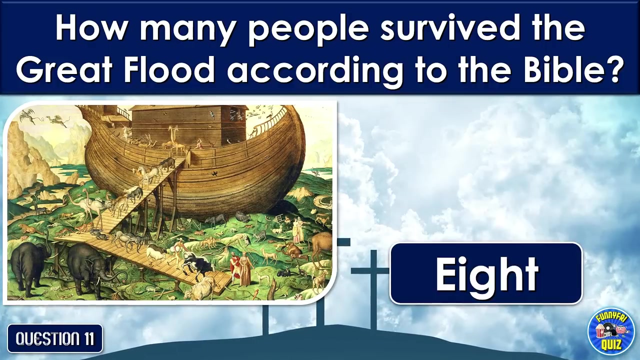 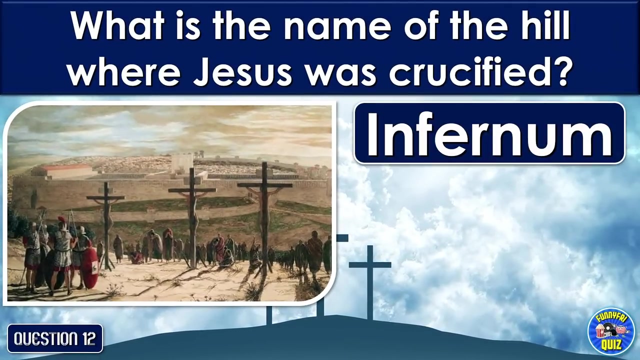 Stephen: Who was Noah's grandfather? Methuselah. How many years did Methuselah live? 969 years Years. He bore a great deal of blood and east of the earth, Moses. How many people survived the Great Flood according to the Bible? 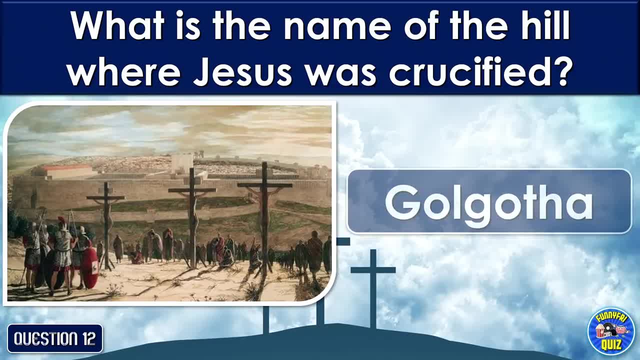 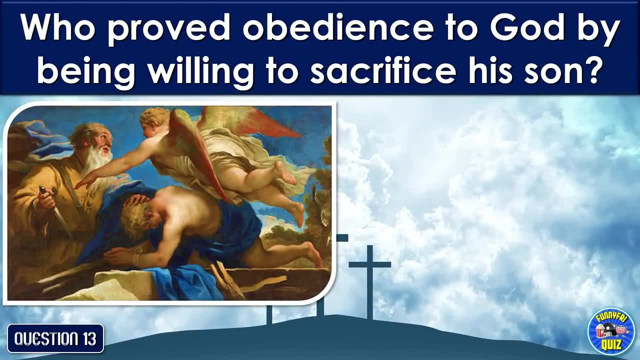 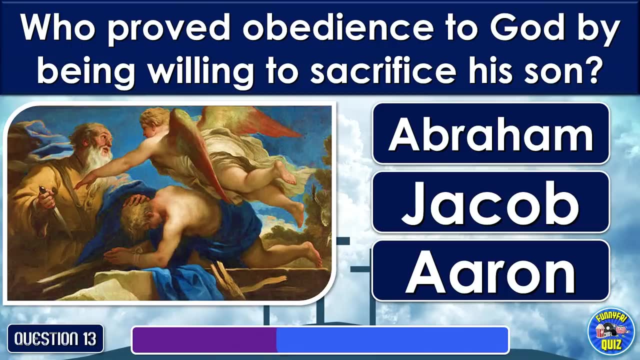 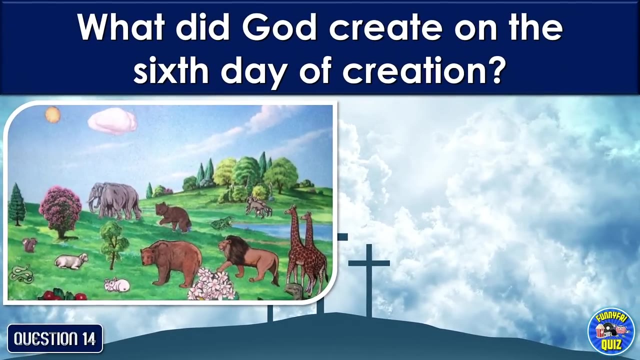 ねぇ Countless partial nervousoma. How many people survived the Great Flood? according to the Bible, Golgotha, who proved obedience to God by being willing to sacrifice his son, Abraham. what did God create on the sixth day of creation? 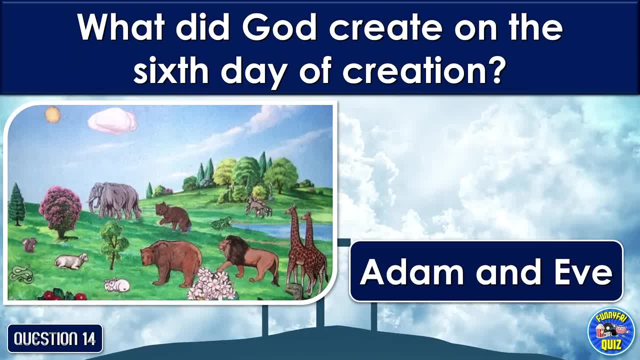 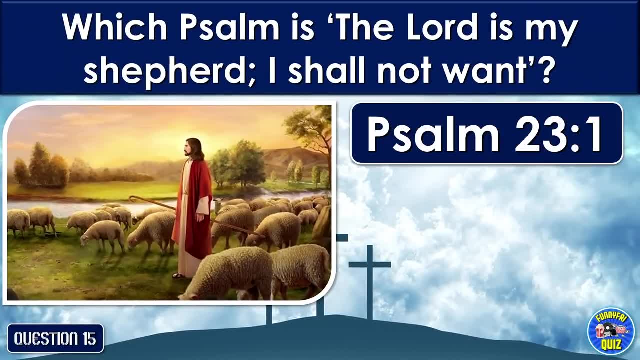 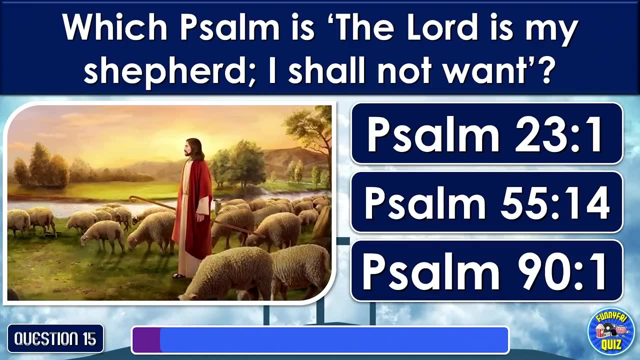 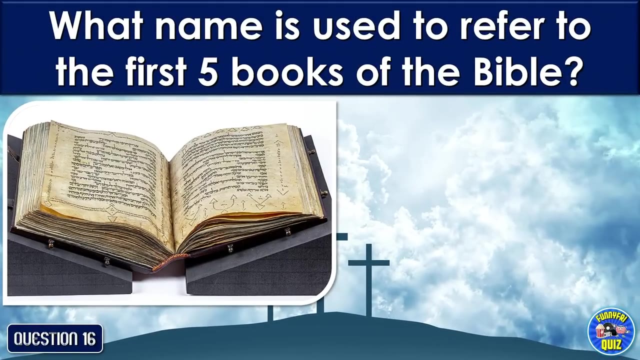 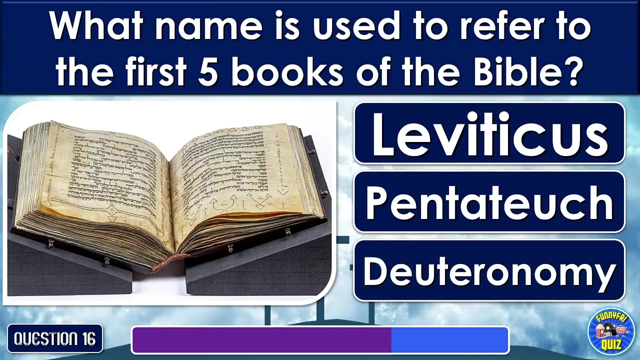 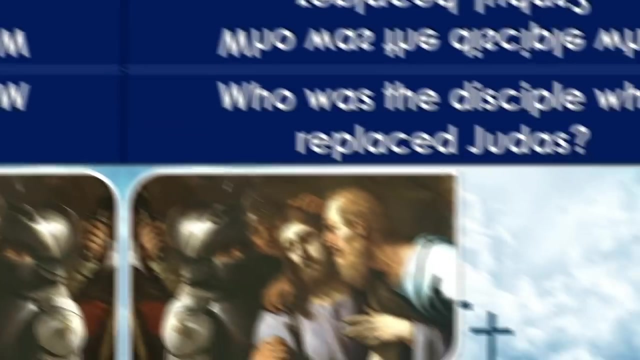 Adam and Eve. which psalm is? The Lord is my shepherd. I shall not want Psalm 23,, verse 1.. What name is used to refer to the first five books of the Bible? The Pentateuch? Who was the disciple who replaced Judas? 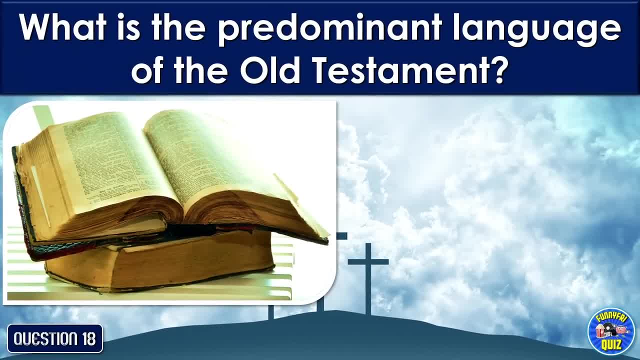 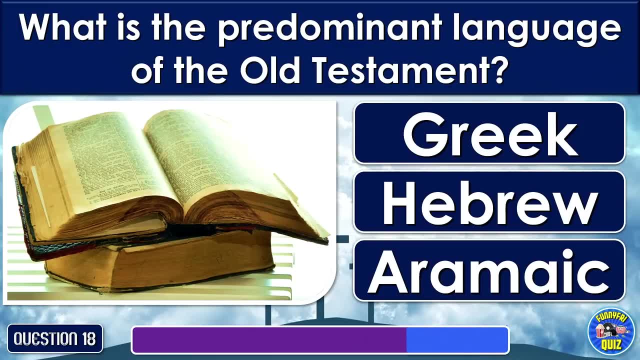 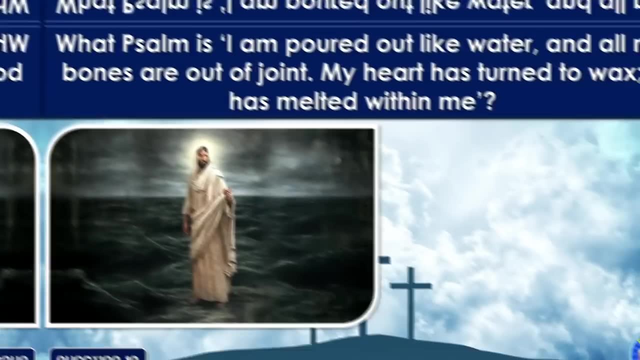 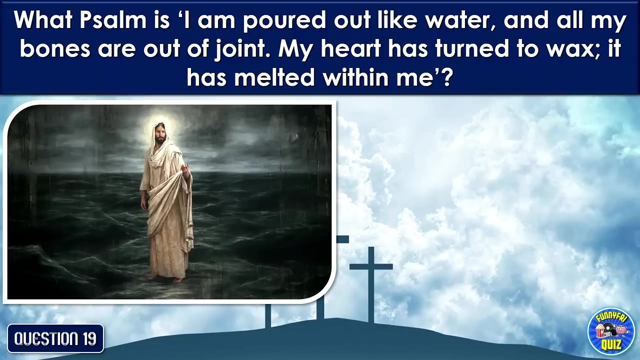 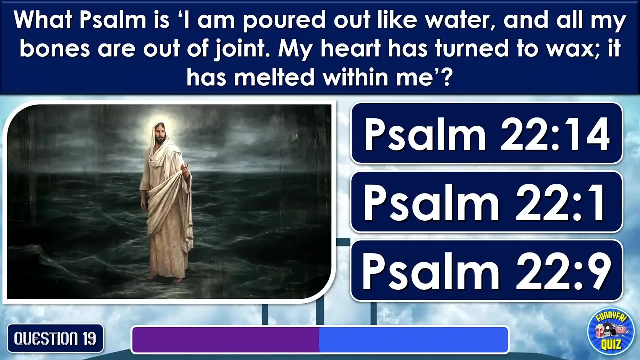 Matthias? What is the predominant language of the Old Testament? The Hebrew? What psalm is? I am poured out like water and all my bones are out of joint. My heart has turned to wax. it has melted within me. Psalm 22,, verse 14.. What name is used to refer to the first five books of the Bible- The Pentateuch? What name is used to refer to the first five books of the Bible- The Pentateuch? What name is used to refer to the first five books of the Bible? 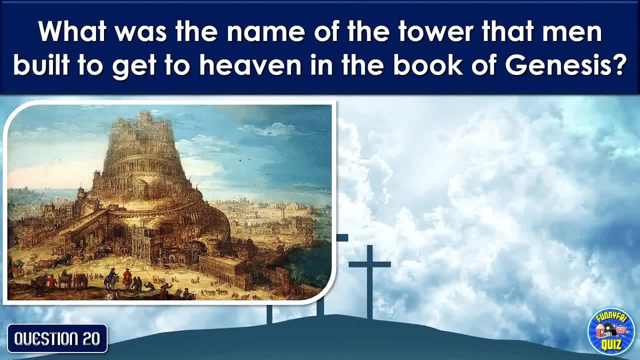 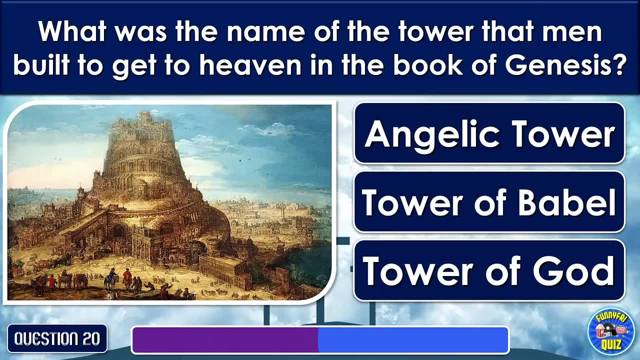 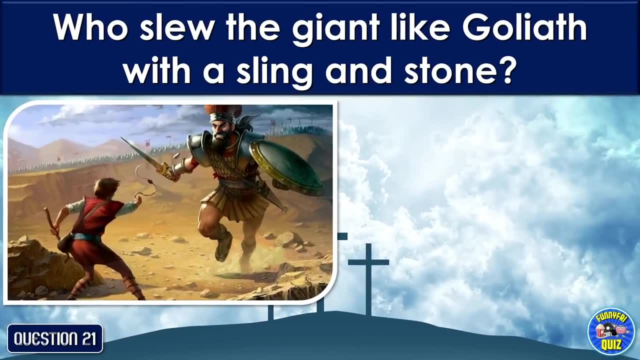 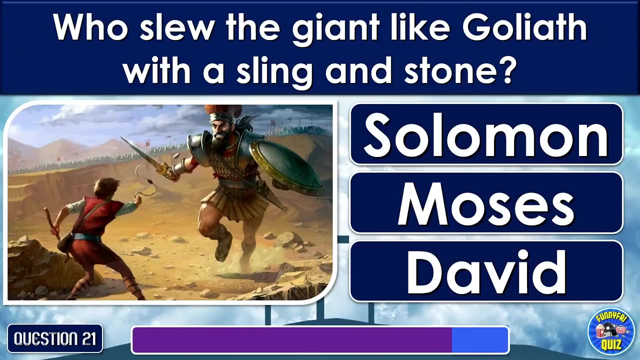 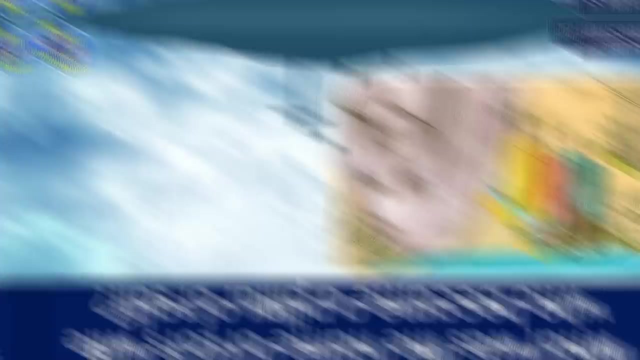 The Pentateuch? What is the name of the tower that men built to get to heaven in the book of Genesis, The Tower of Babel. Who slew the giant like Goliath with a sling and stone? David, David. What was the name of Lot's wife, who became a pillar of salt? 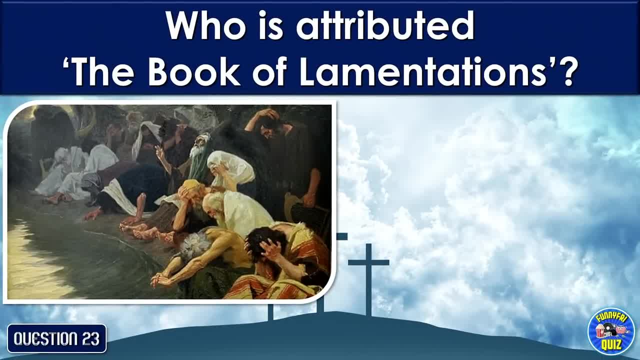 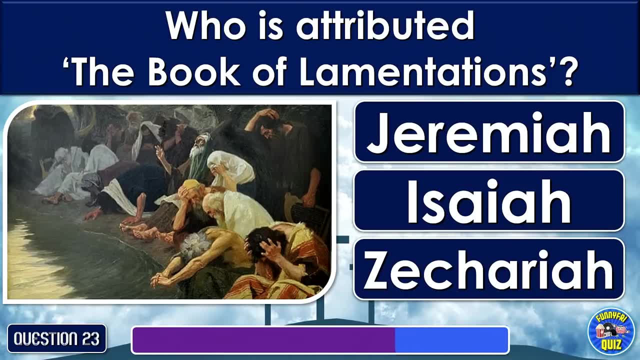 Adu or Edith, Who is attributed the book of Laman, A woman on the mount of Enoch, Or a woman on the mountain of Noah Who is added to the projectile and purgatory of the temple, The prophet Jeremiah. 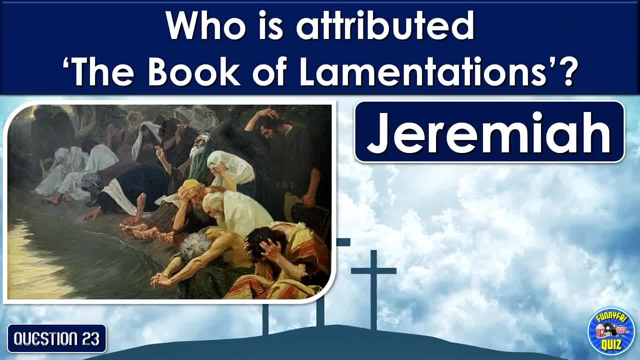 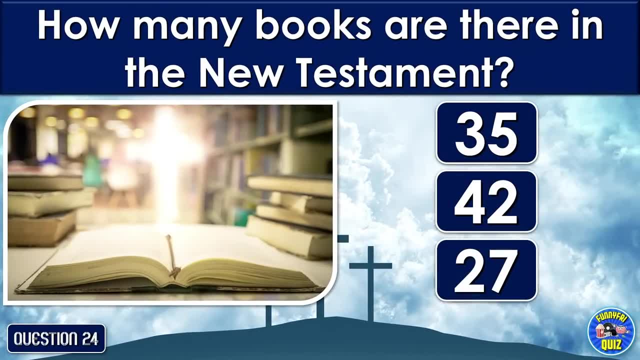 Who? The judgmental deity or a tapes عن an impure beast. aat The perchonite temple or the temple of the sun Beaticius his виua boy What is the name of the name of these three languages? � Jeremiah. 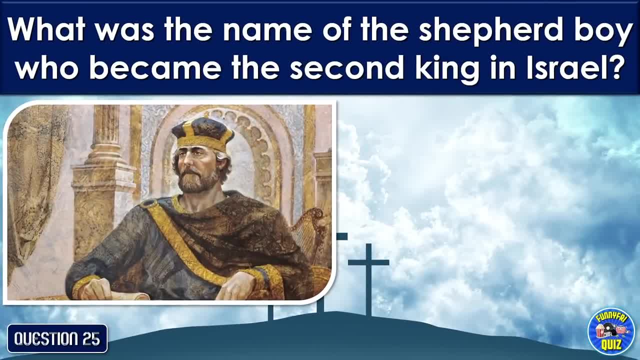 How many books are there in the New Testament? Sheseh, Jeremiah. How many books are there in the New Testament, Jeremiah? How many books are there in the New Testament? She climate? How many books are there in the New Testament? Twenty-seven, Twenty-seven.